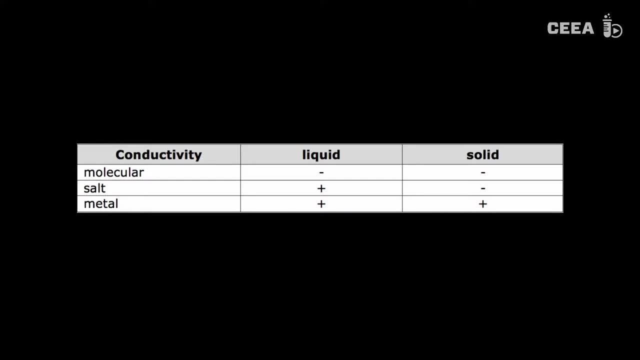 the valence electrons moving freely through the crystal. A salt consists of ions. In the crystal lattice, positive and negatively charged ions are organized alternately in such a way that the salt crystal as a whole is electrically neutral. A molecular substance consists of neutral molecules. 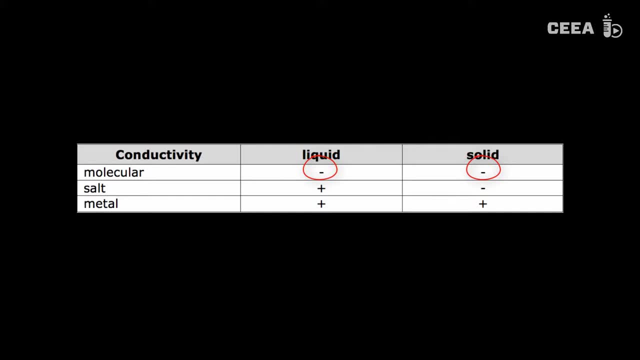 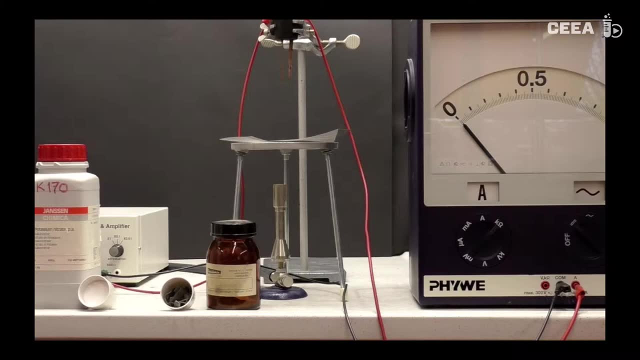 As a rule, there is no transport of electrical charge between the individual molecules. Let us check the foregoing statements by some simple experiments. How traditional a metal lattice works. All we need is an electrical power source, a set of cables, a heat-resistant beaker and an ammeter. 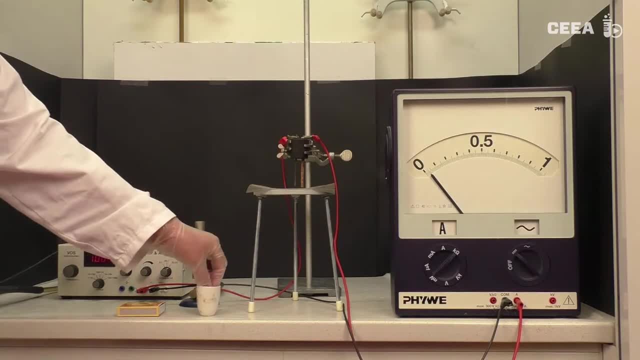 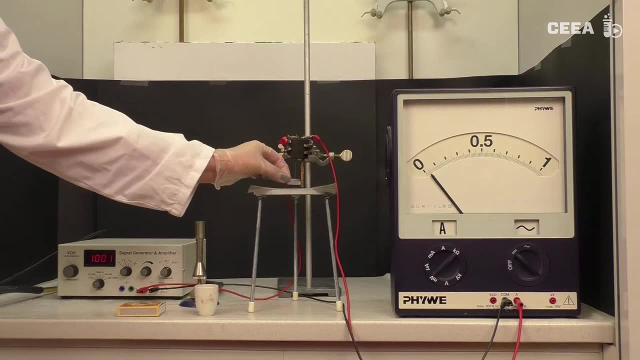 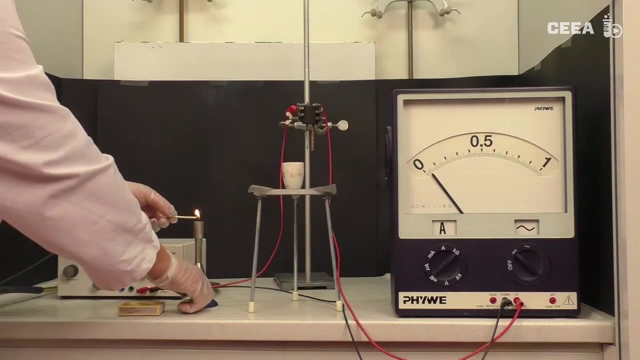 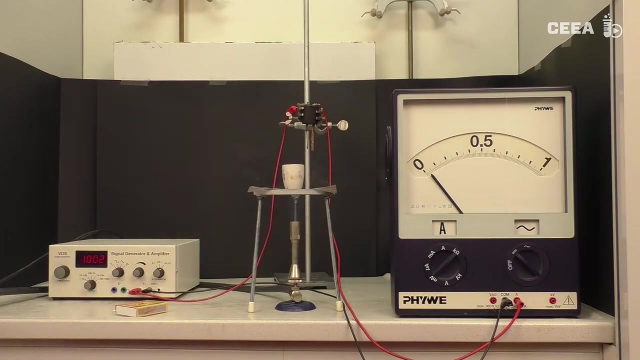 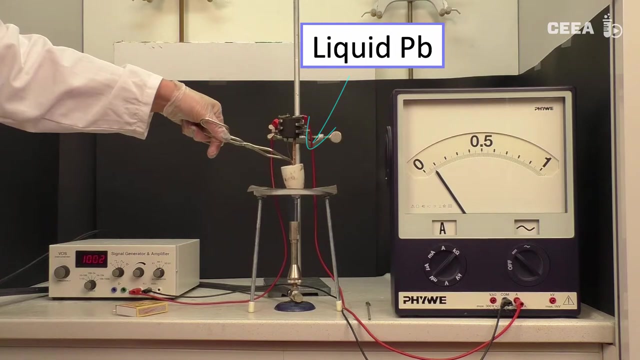 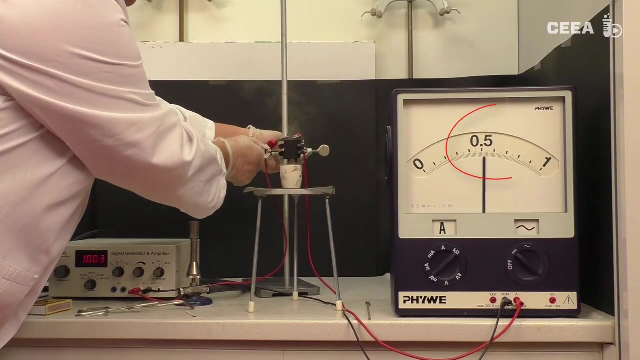 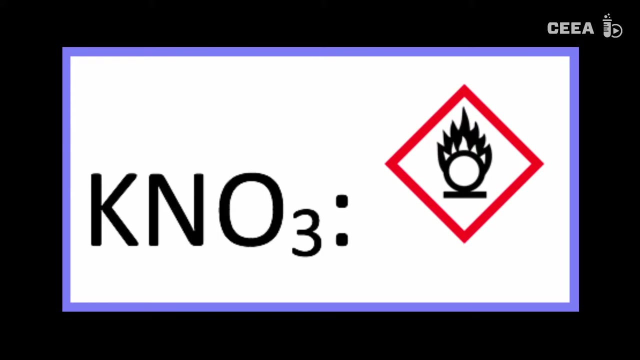 We start with a piece of lead. The ammeter clearly shows that solid lead conducts electricity. How to melt the lead? When we melt the lead, We observe that in the liquid phase, lead also conducts electricity. We repeat the experiment with a salt, potassium nitrate. 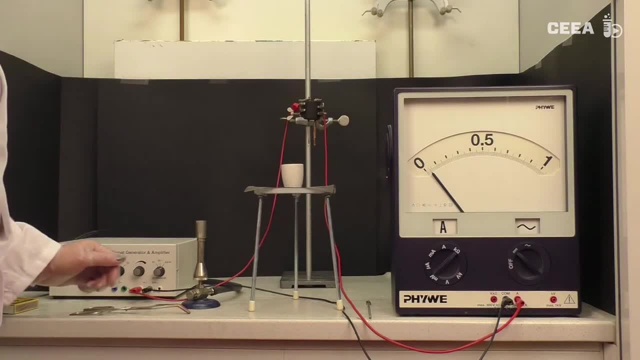 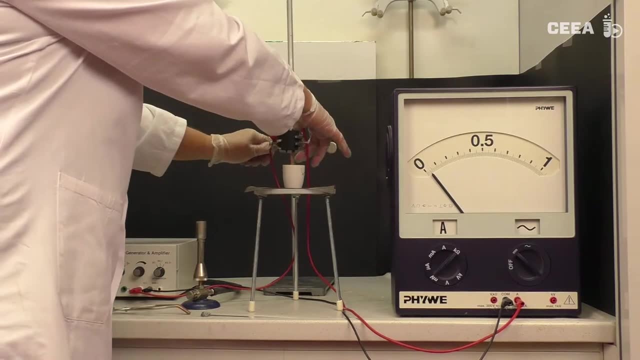 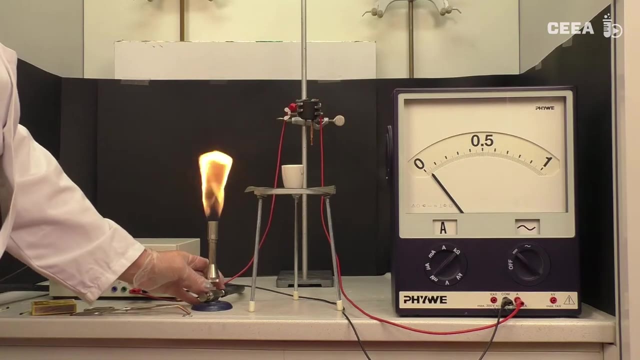 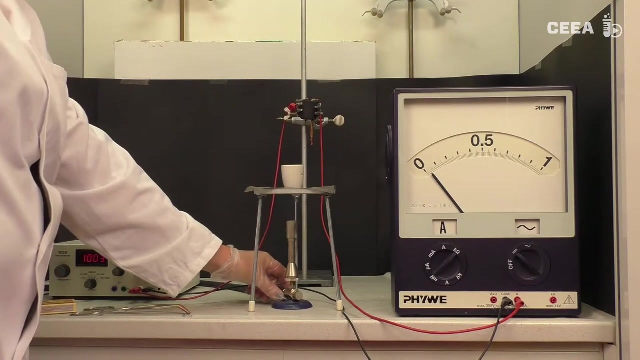 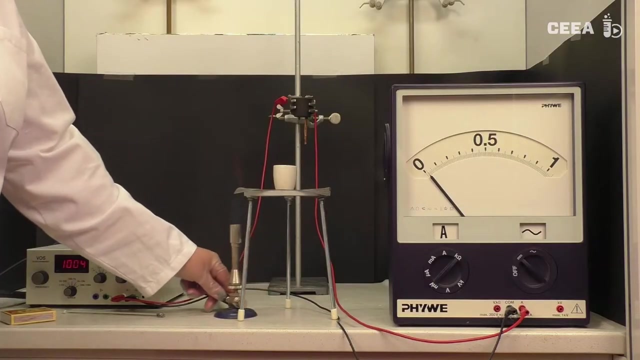 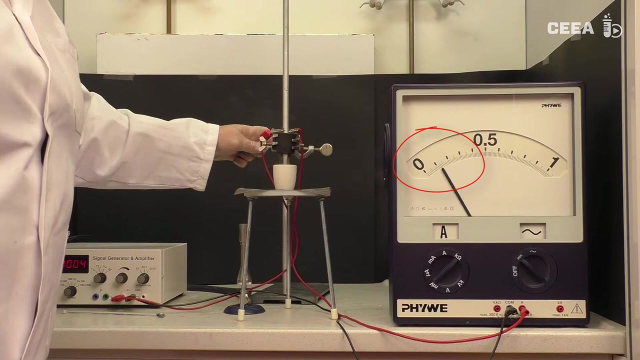 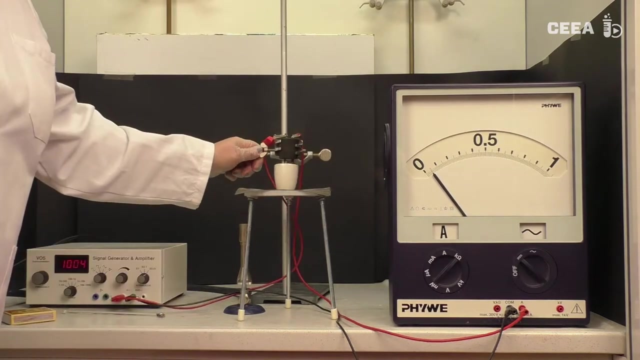 There is no sign of conductivity, although the salt crystals contain plenty of charged particles. Now let's see what happens upon melting. This takes some time because the salt melts at 607 K. And what do we observe Upon melting? the salt appears to be a conductor. Finally, we investigate the reaction. We observe that in the liquid phase lead also conducts electricity. We repeat the experiment with a salt: potassium nitrate. There is no sign of conductivity, although the salt crystals contain plenty of charged particles. There is no sign of conductivity, although the salt crystals contain plenty of charged.